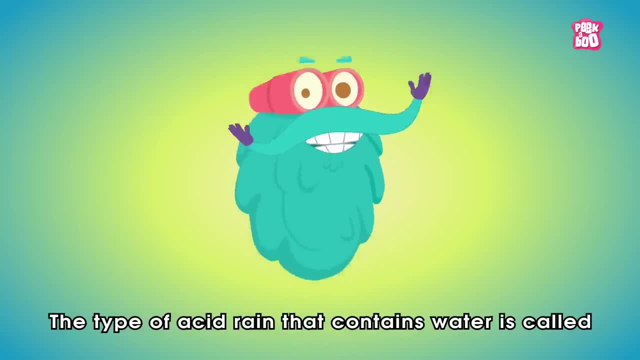 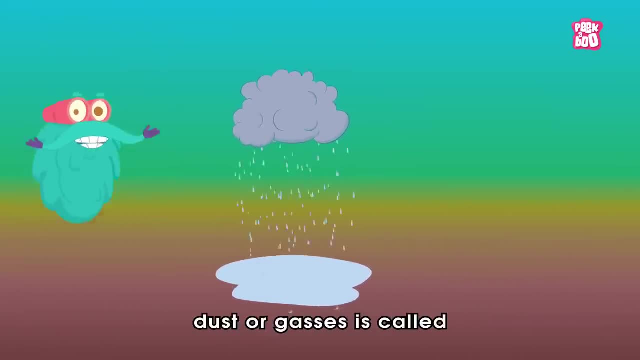 The type of acid rain that contains water is called wet deposition. Whereas acid rain formed with dust or gases is called dry deposition. 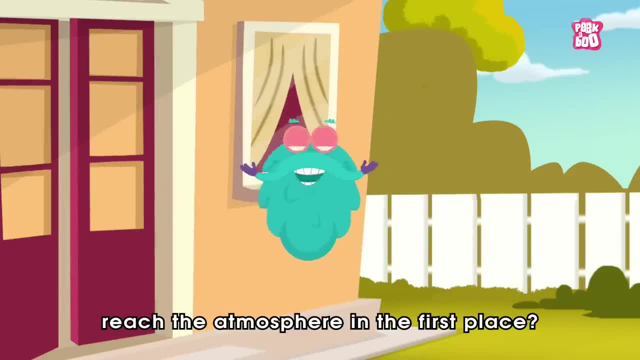 But how do these gases reach the atmosphere in the first place? Well, there are two main sources for it. 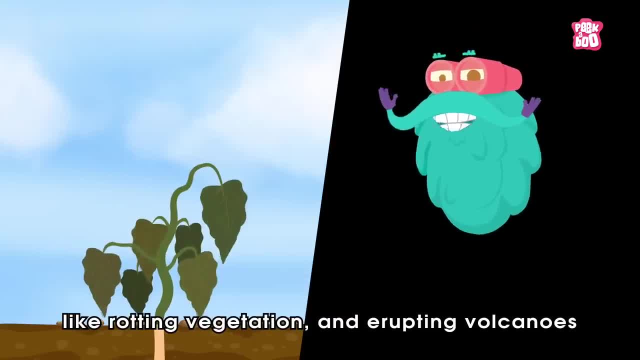 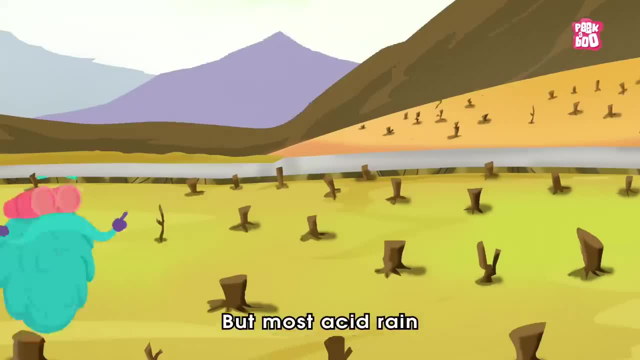 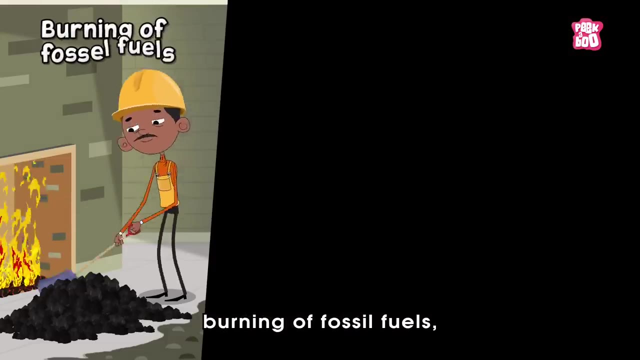 First is the natural source like rotting vegetation. And erupting volcanoes release some chemicals that can cause acid rain. But most acid rain is a product of human activities like burning of fossil fuels.. 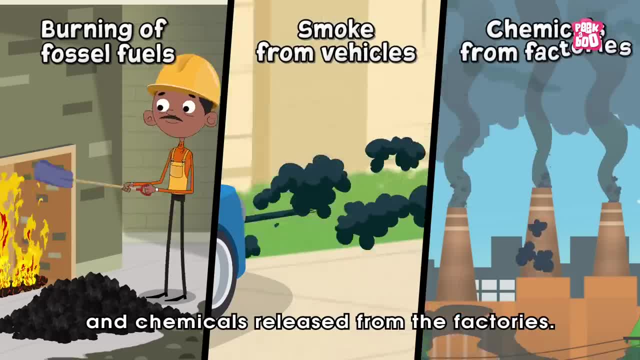 ..smoke coming from vehicles and chemicals released from the factories. 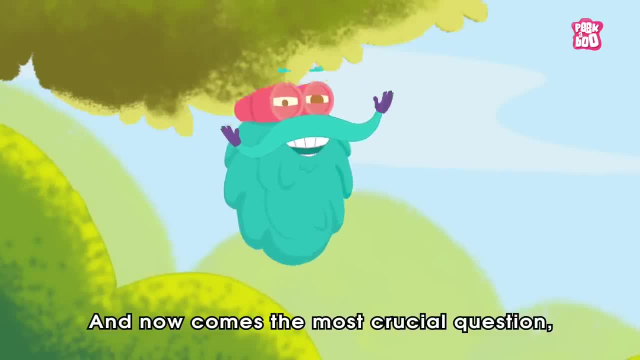 And now comes the most crucial question and that is.. ..what causes the rain to turn acidic? Well, it's important to understand that normal rain is already a little acidic. Yes, my friends. 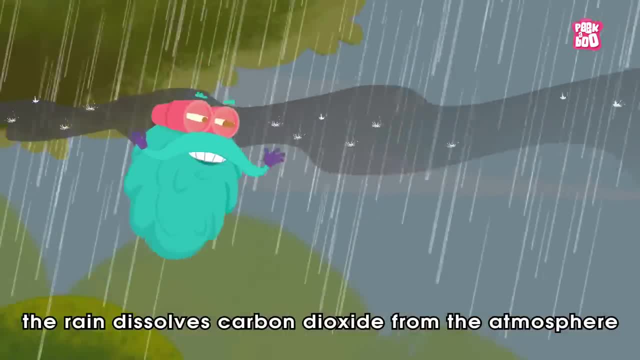 While falling towards the ground, the rain dissolves carbon dioxide from the atmosphere.. 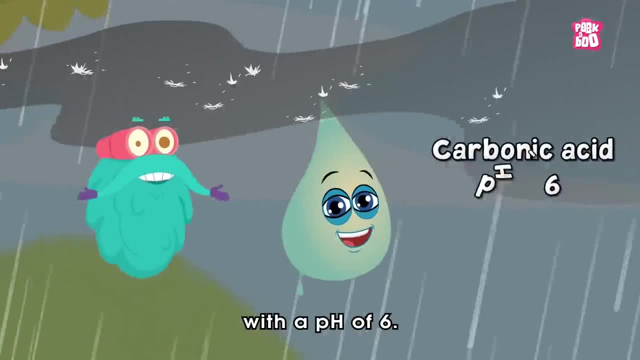 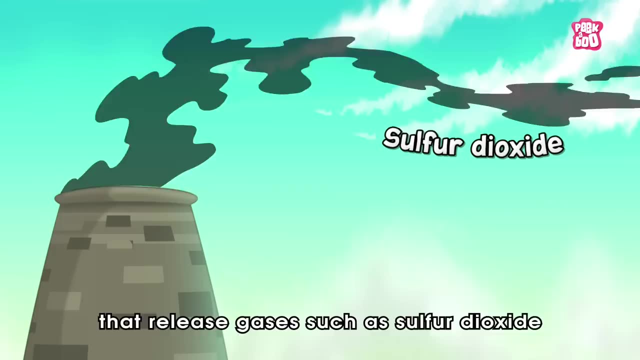 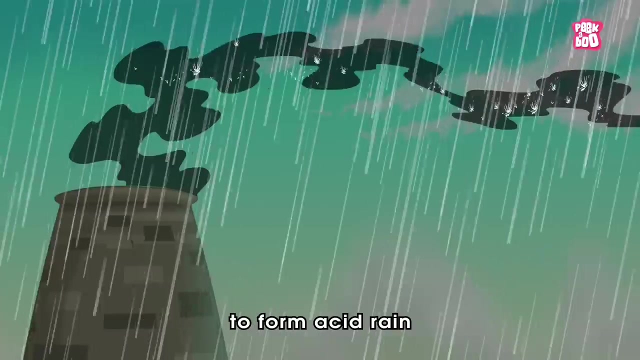 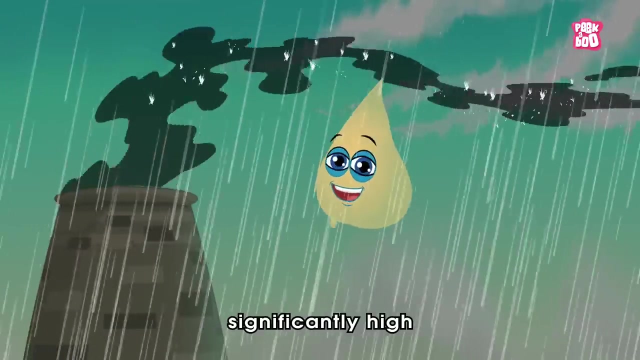 ..that forms carbonic acid with a pH of 6. But when we burn fossil fuels that release gases such as sulphur dioxide.. ..and nitrogen oxide, a much stronger acid, gets into our rain.. ..to form acid rain with pH 3 which increases the acidity of rain significantly high. Still confused? 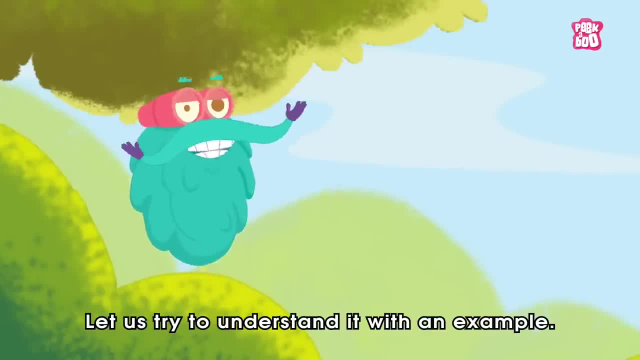 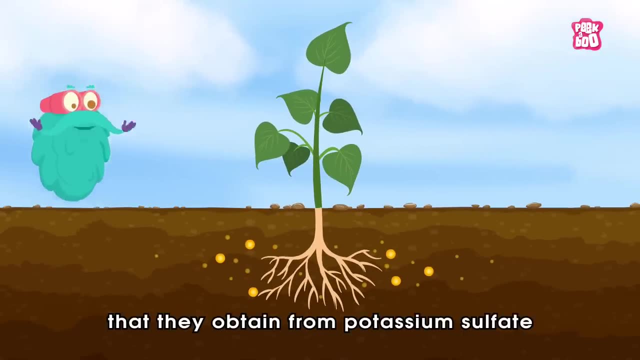 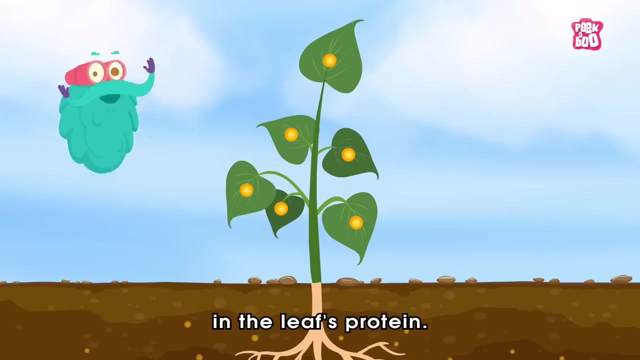 Okay, let's try to understand it with an example. You see, plants intake some sulphur to grow that they obtain from potassium sulphate. This is already present in the soil. The sulphate is consumed through the roots as the sulphur atoms bond with carbon atoms in the leaves' protein. 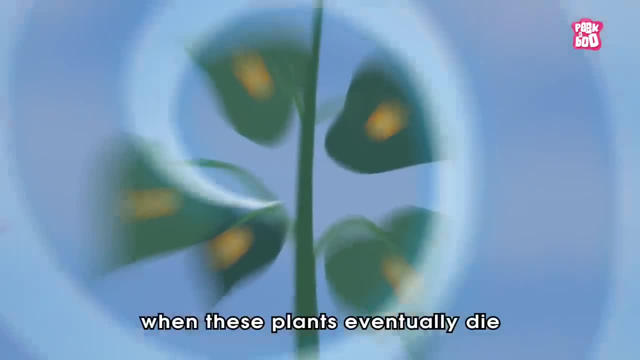 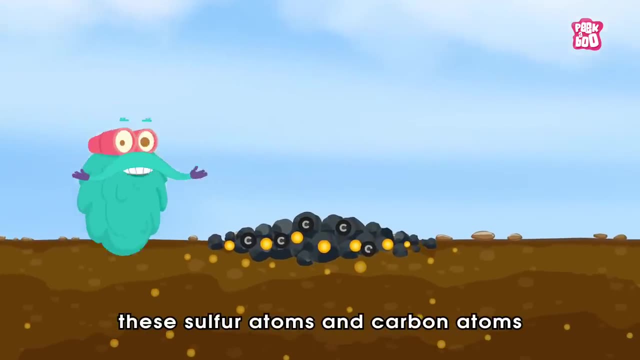 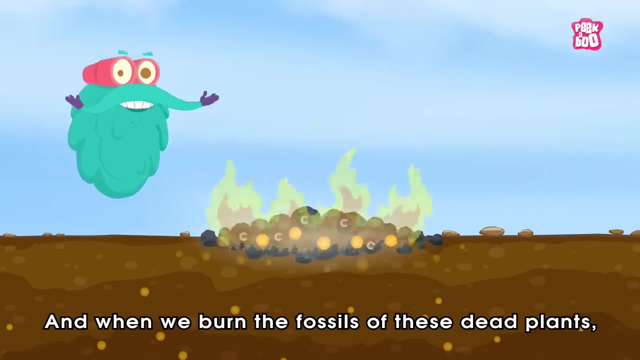 And after millions of years, when these plants eventually die and turn into coal.. ..these sulphur atoms and carbon atoms remain intact. And when we burn the fossils of these dead plants.. ..the sulphur and carbon atoms mix with the oxygen in the air.. ..and are released into the atmosphere as sulphur dioxide and carbon dioxide. 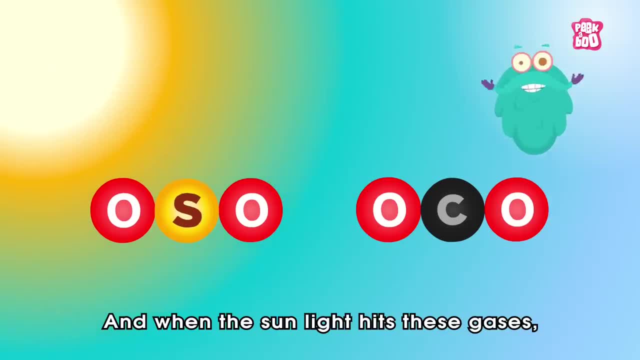 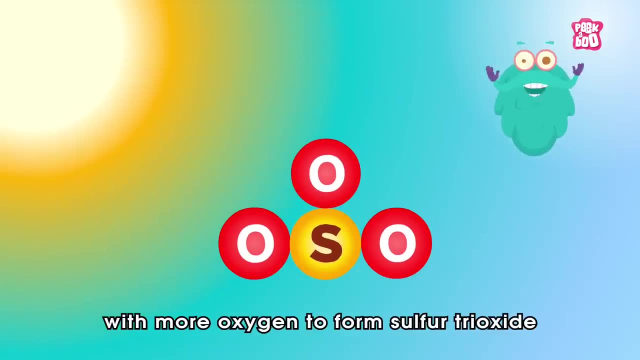 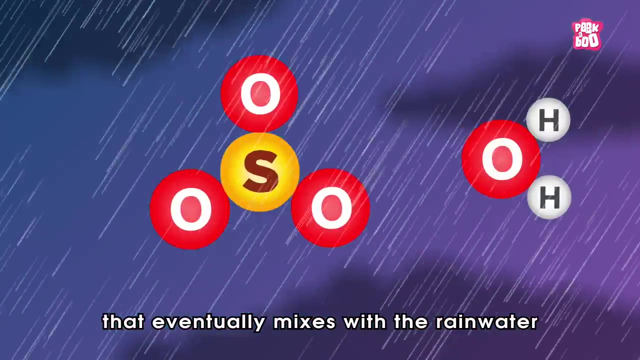 And when the sunlight hits these gases, a chemical reaction takes place.. ..where the sulphur dioxide reacts with more oxygen to form sulphur trioxide. That eventually mixes with the rainwater to create sulphuric acid. 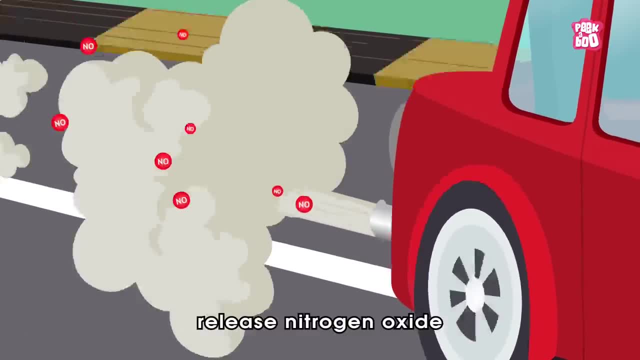 Similarly, when our vehicles release nitrogen oxide into the atmosphere.. 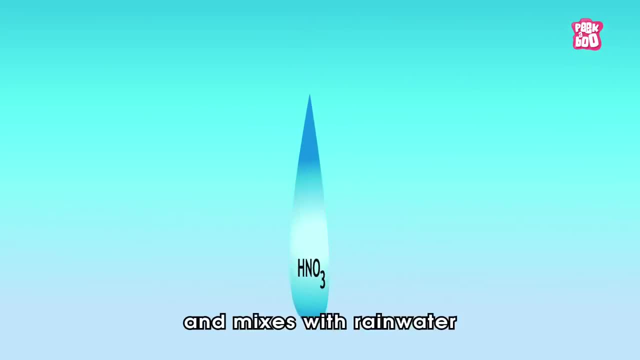 ..they react with more oxygen and mixes with rainwater to form nitric acid. 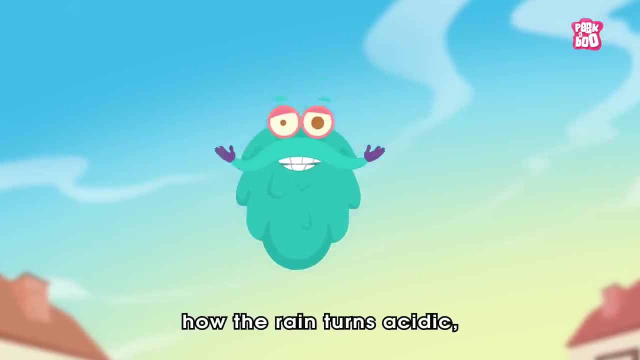 And now we know how the rain turns acidic. So, let us now learn its effect on our environment. 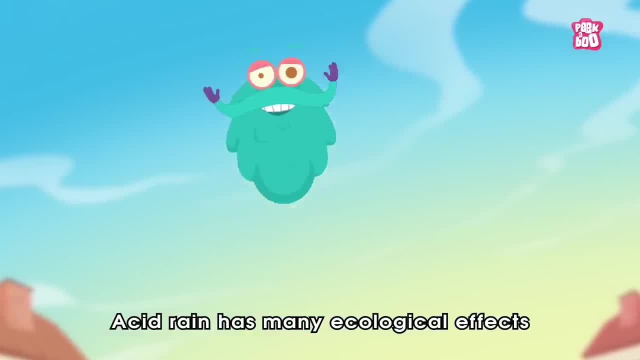 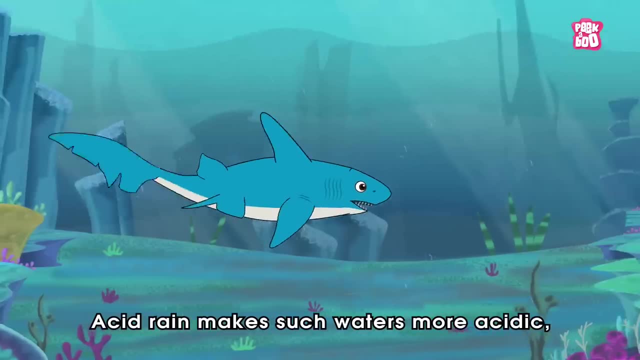 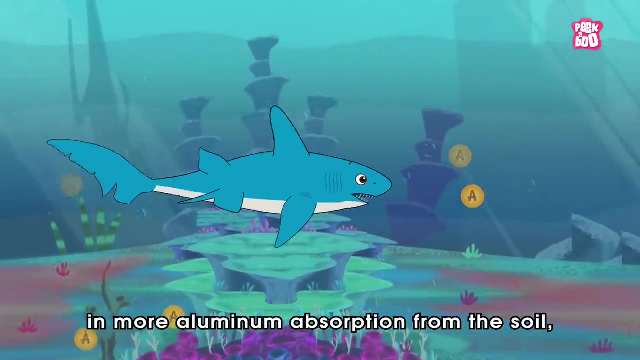 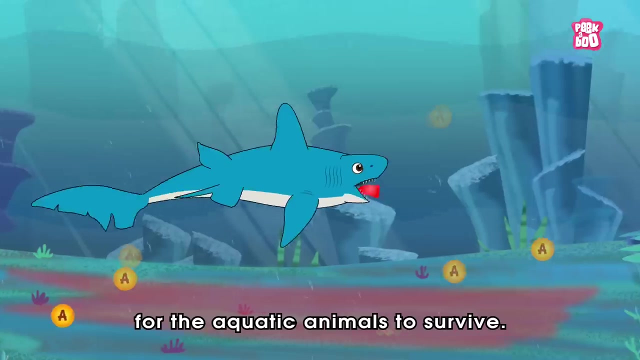 Acid rain has many ecological effects, primarily on lakes, rivers and other aquatic environments. Acid rain makes such waters more acidic, which results in more aluminum absorption from the soil.. ..which is carried into lakes and rivers.. ..making the water toxic for the aquatic animals to survive. 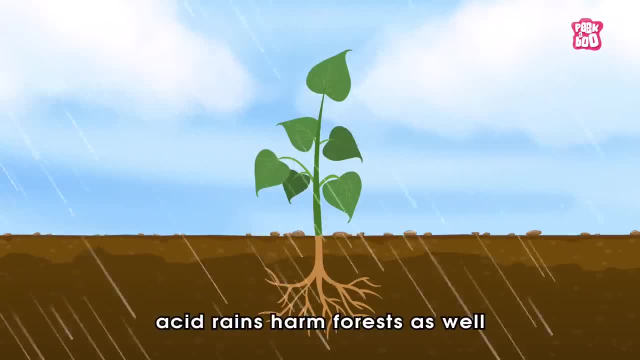 Not only that, acid rains harm forests as well.. ..by damaging leaves and robbing the soil of essential nutrients.. 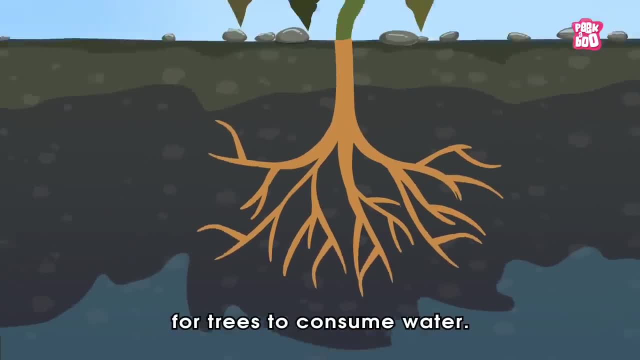 ..and making it difficult for trees to consume water. 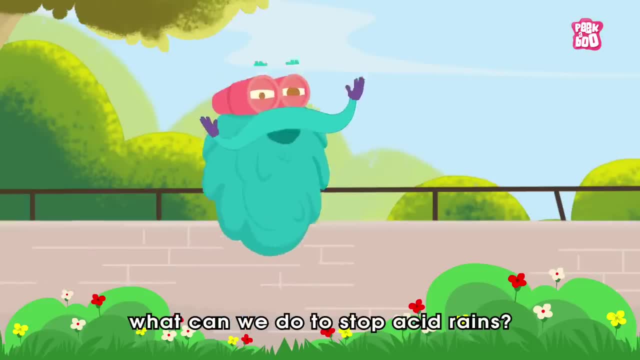 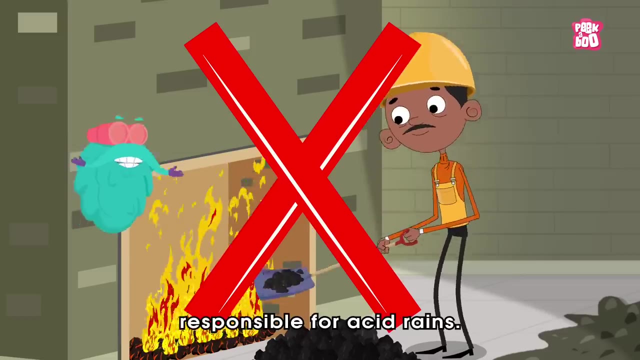 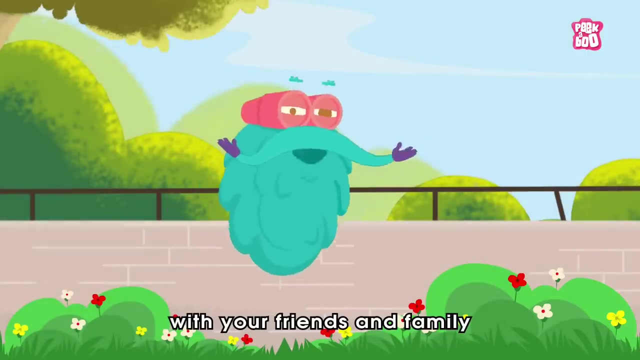 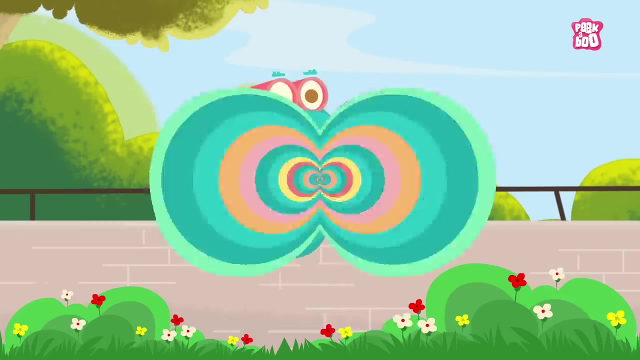 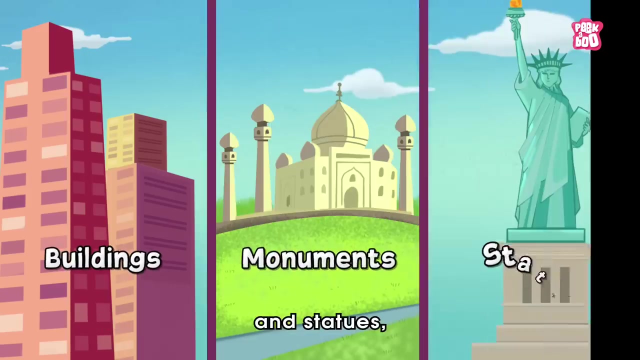 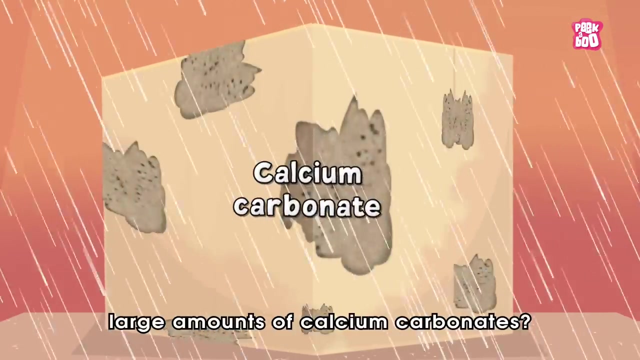 So, now the main concern is, what can we do to stop acid rains? Well, the one easy step we can take is just reducing the burning of fossil fuels. That will decrease the number of pollutants responsible for acid rains. And the next thing is to share this video with your friends and family.. ..to spread awareness about it, as we now feature Trivia Time! Did you know, acid rain damages buildings, monuments and statues? Especially those made of limestone and marble, as they contain large amounts of calcium carbonates. The calcium compounds react with the acid in the rain, damaging them. 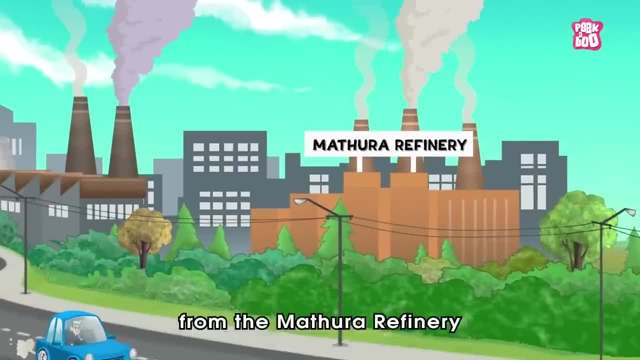 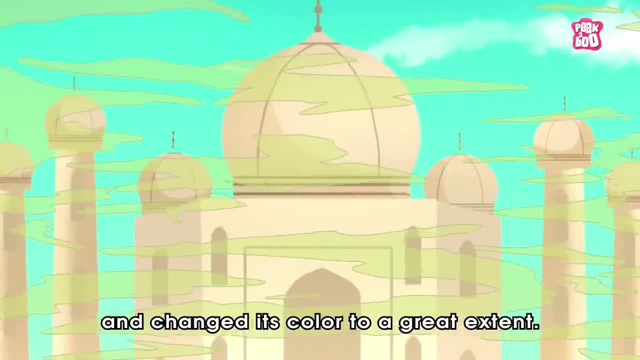 Yes, exhaust gases from the Mathura refinery greatly affected the Taj Mahal at Agra.. ..and changed its colour to a great extent. Hope you enjoyed today's episode.